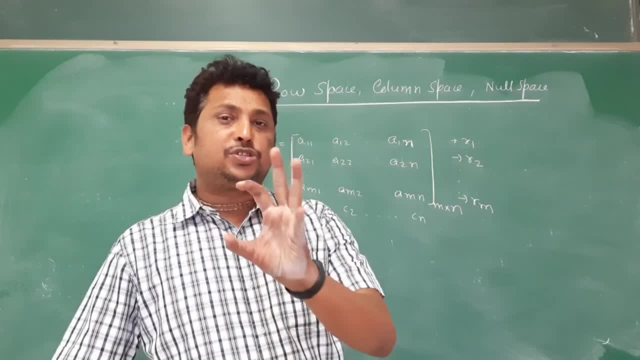 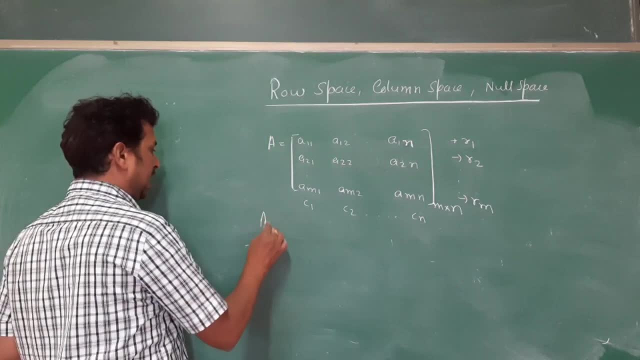 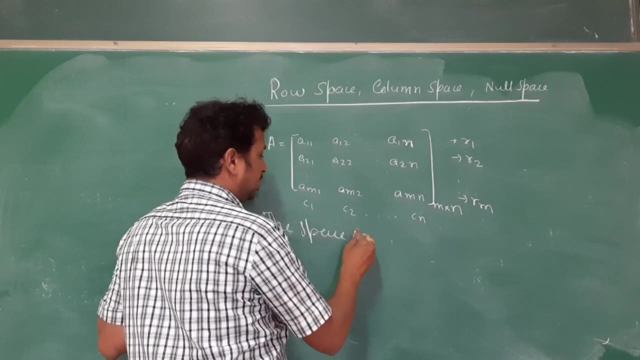 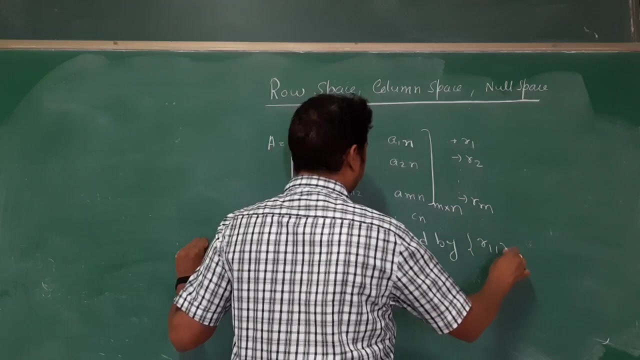 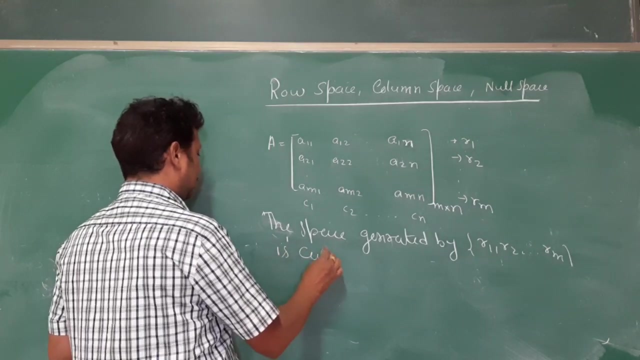 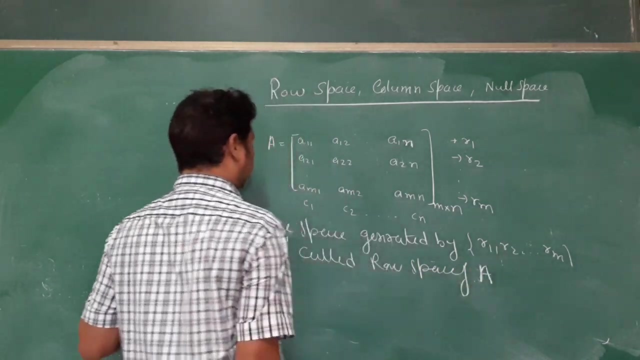 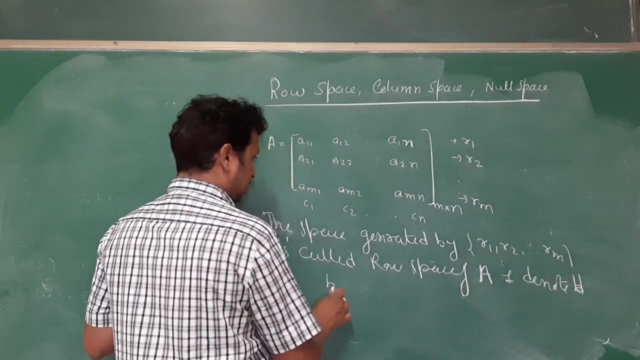 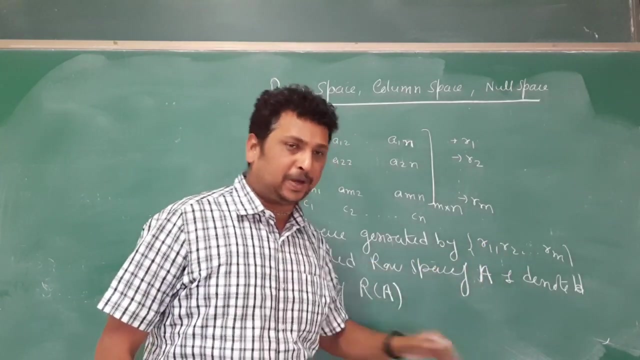 Now any space which generated by these rows is called row space. So any space now that space, that space generated by R1, R2, R3 is called row space of A And it is denoted by R. So how we calculate, I will explain. 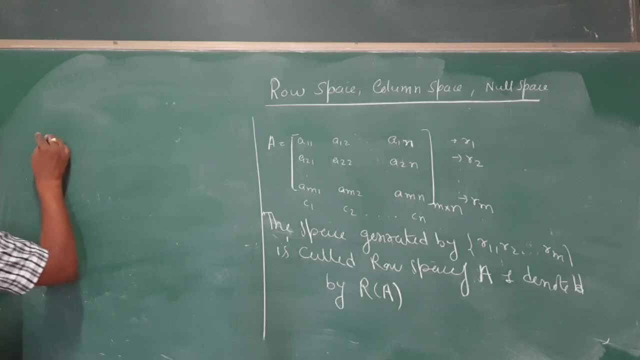 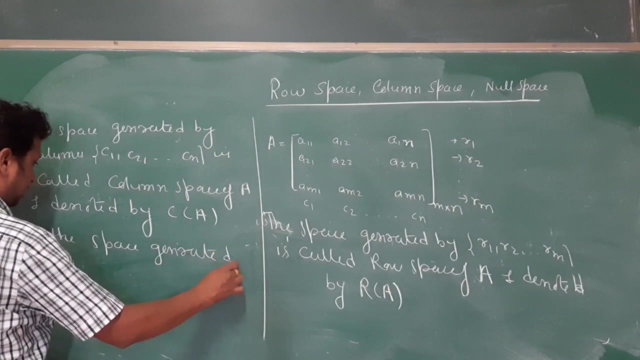 Like. what is column space? The space? let space be matrix space or subspace. The space generated by column space is called column space of A and denoted by R. A linear matrix, N, is given by column space of C. A linear matrix can also be denoted by column space of R. 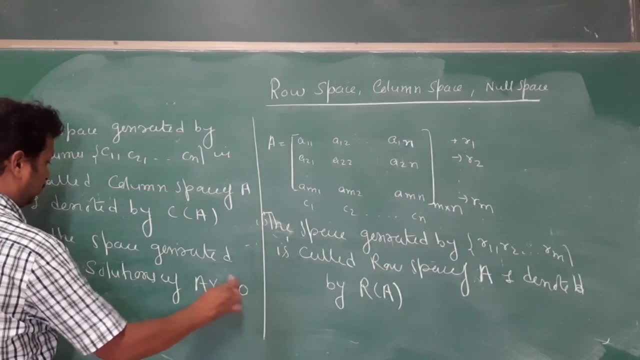 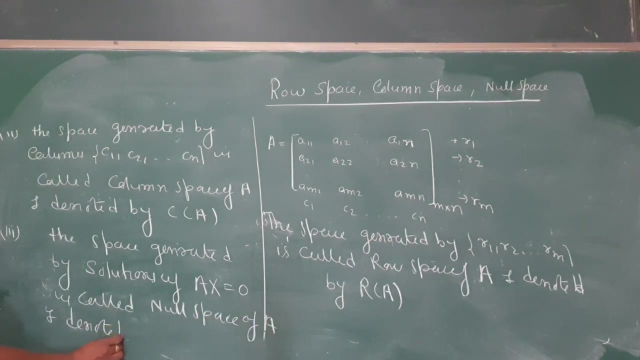 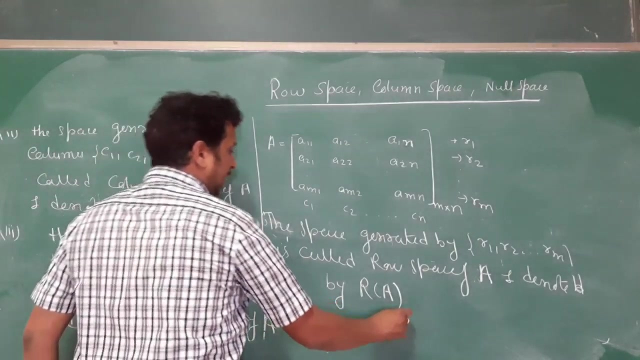 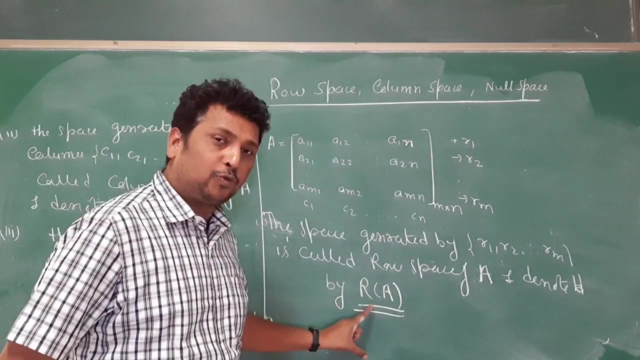 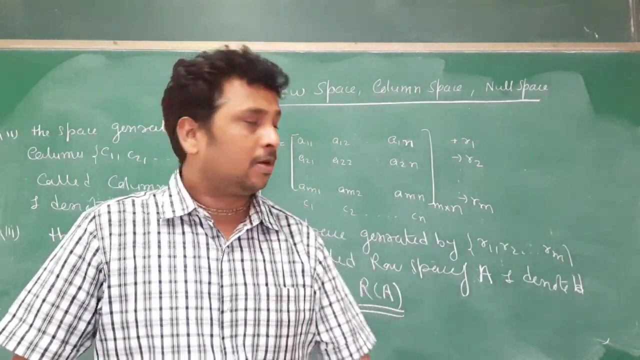 So for a given magnet, see, you have to calculate row space, column space and null space. and the order of calculation is: first we calculate row space and then we write the vectors which generates row space, then we go for null space and then we write column space. 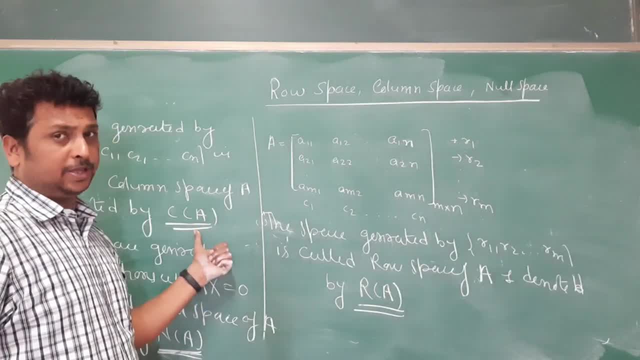 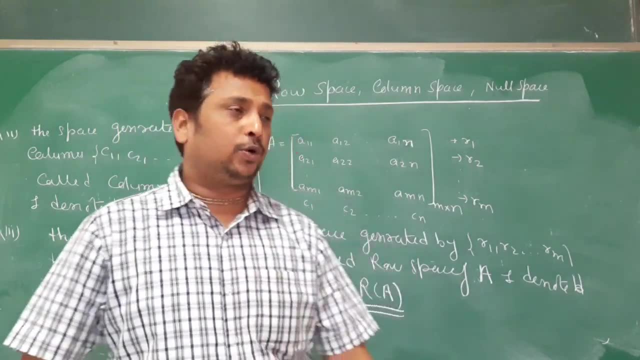 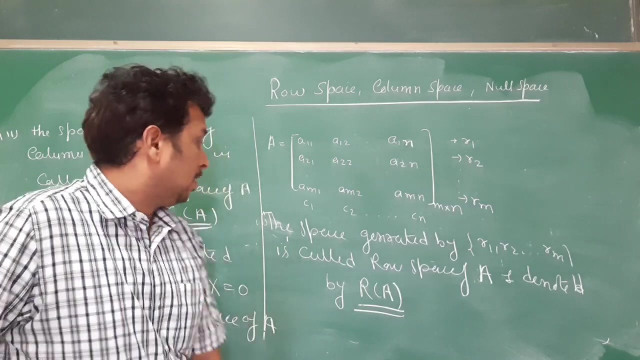 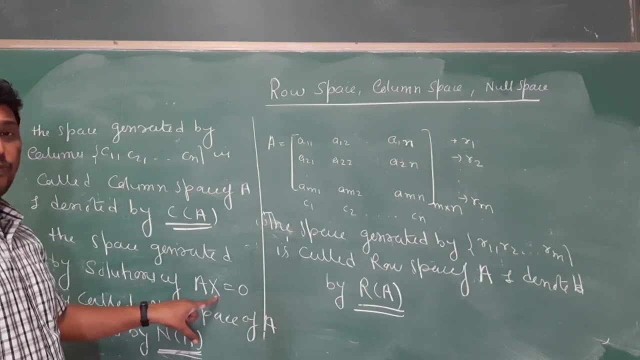 Dimension of row space is equal to dimension of column. space means how many elements are there. in basis of R, A is always equal to dimension of column A. Null space is separate. null space means the solution of AX is equal to 0, or sometimes what we are doing, we are reducing A into a glum form to calculate row form. row space. 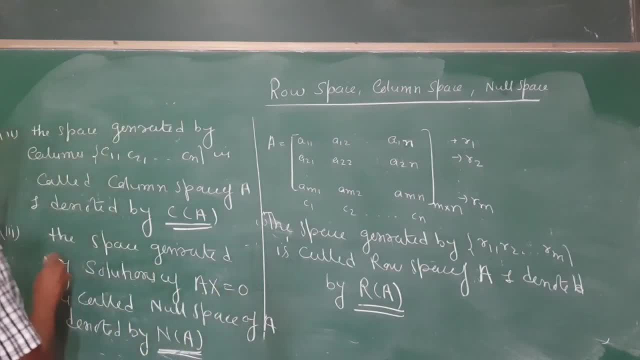 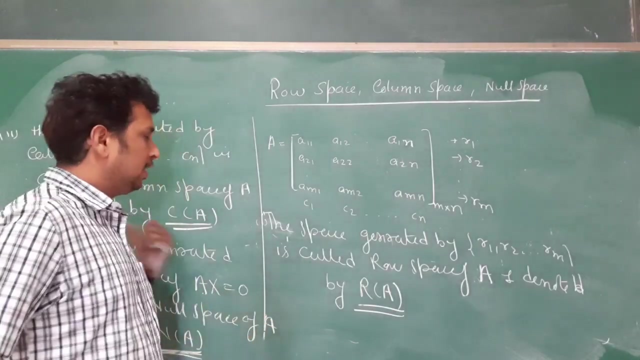 in that we are telling either solution of AX is equal to 0 is same like solution of UX is equal to 0. Because row glum form is upper type of magnet, so you do here upper type of magnet. so either you find solution of this or this. both are same. so that is easy for us, so we can calculate. 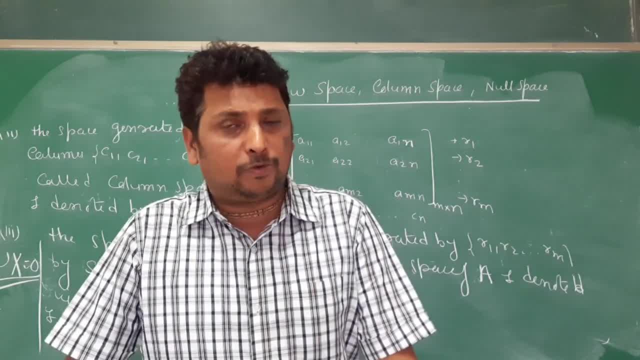 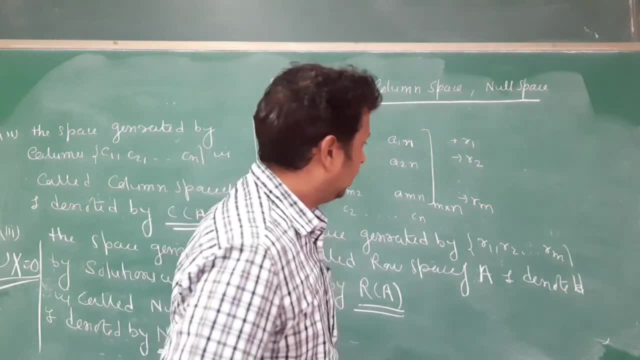 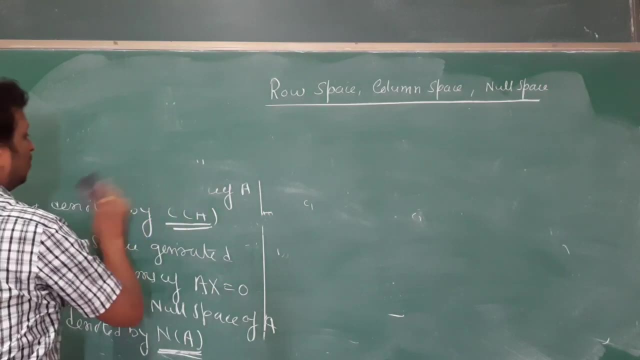 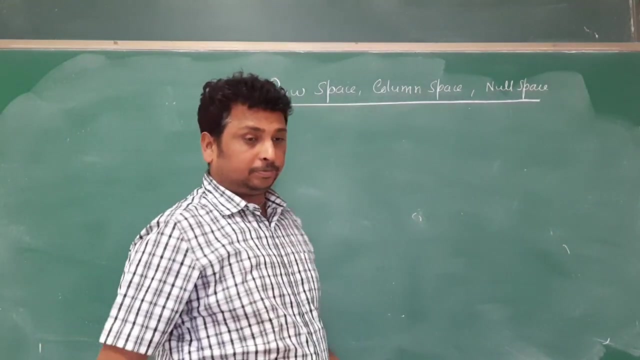 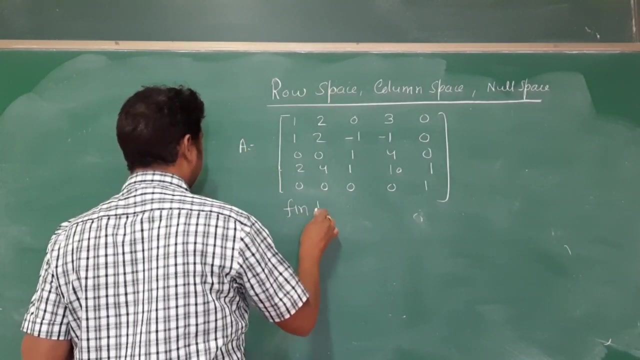 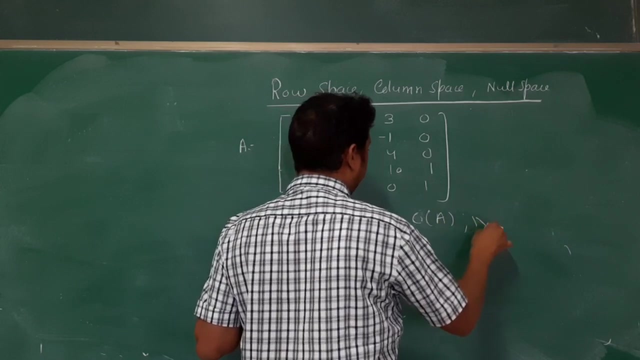 space generated by solution of that, that is, null space. How we calculate, I will explain in this lecture, only don't worry. so we will start with one problem. This problem is very important because it is so many examples. Enter I here, N, and then I will see. 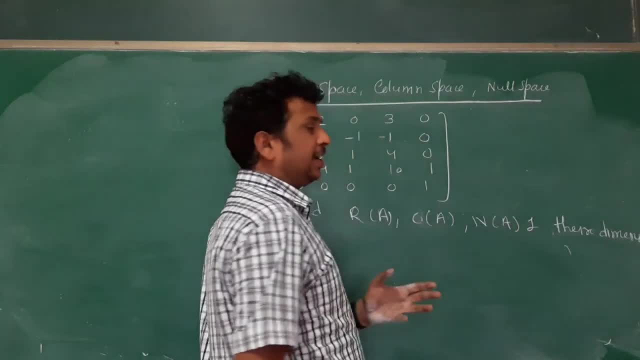 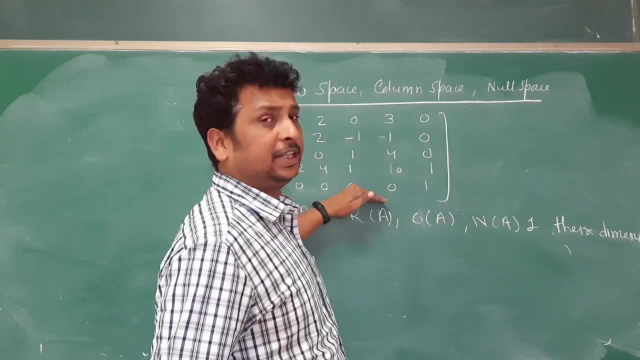 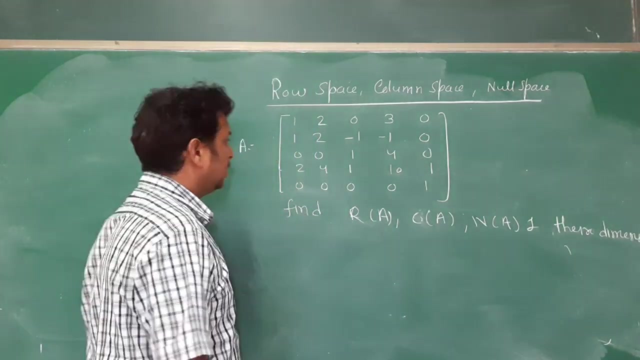 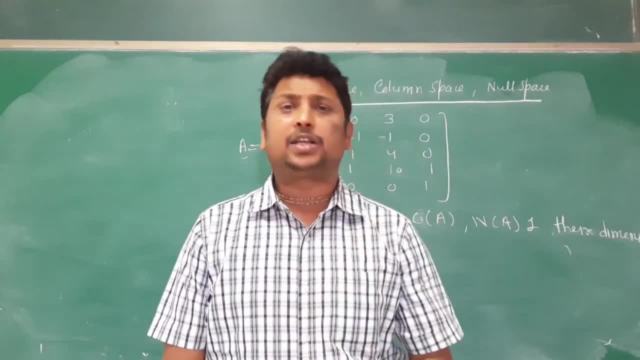 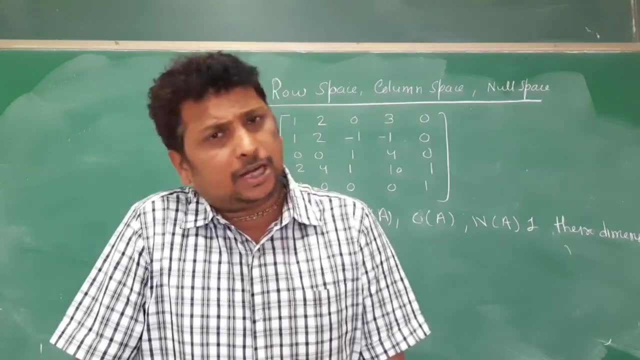 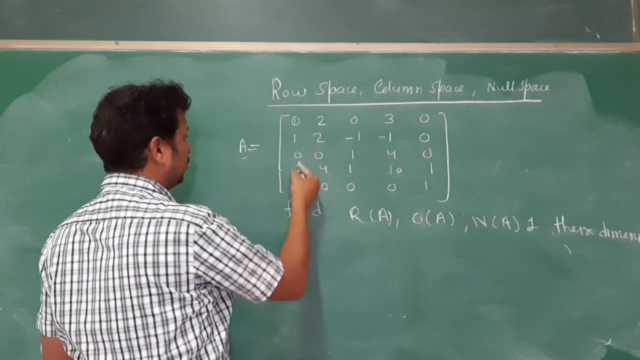 step wise process. first step is convert this given matrix into echelon form: row, echelon form, Whatever given matrix. So this is the first step. So this is the first step: Convert this into echelon form. What is it again from first? make this identity one. it is there. make this one 0. this one 0. 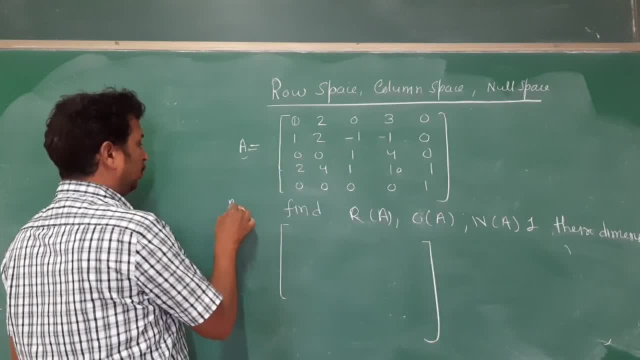 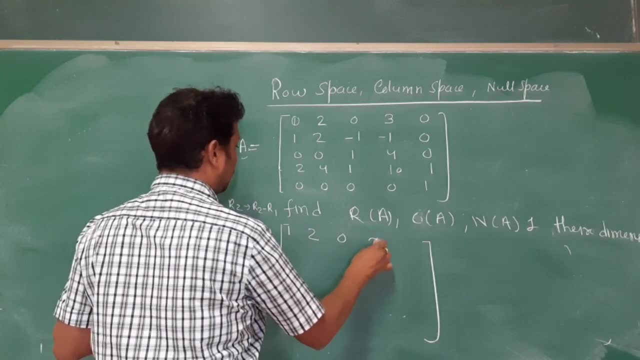 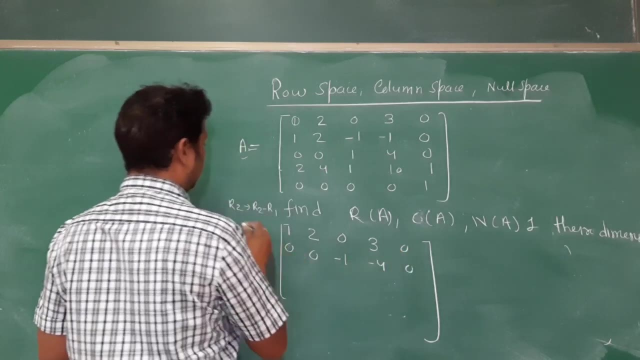 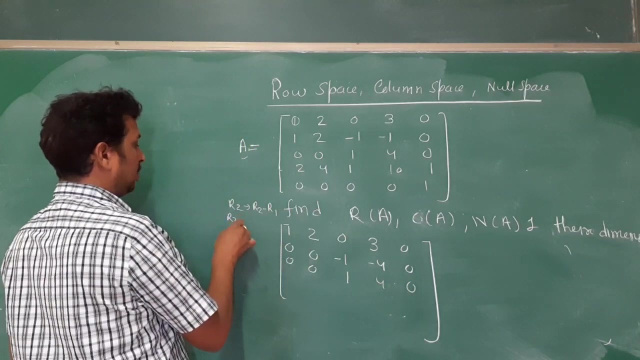 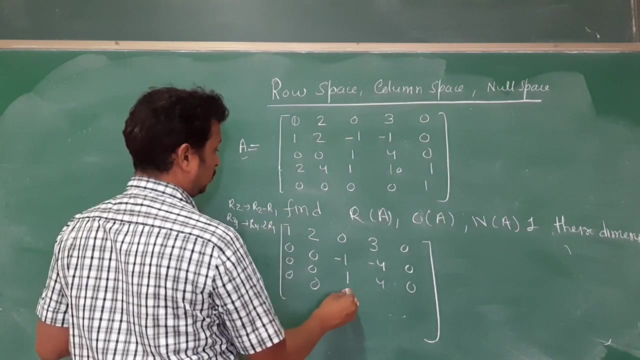 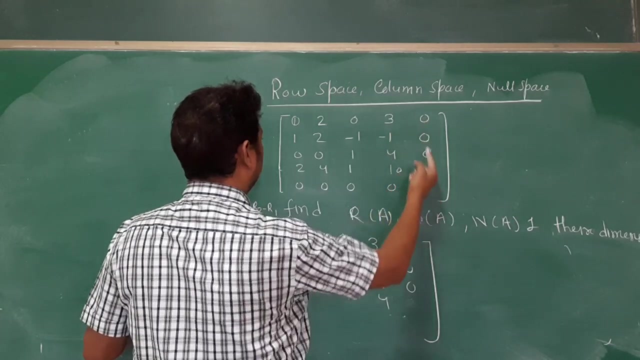 means all entries below that 0.. So what we are doing to R2, change to R2 minus R1, 0, 0 minus 1 minus 1, then this is already 0.. So this is 0.. So R4, R4 minus 2R, So it is 0, 0, 1, 4, 1.. 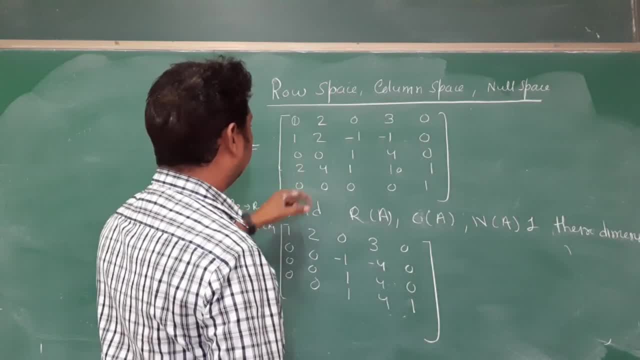 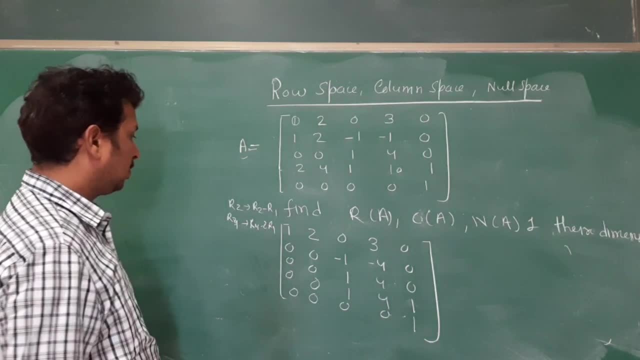 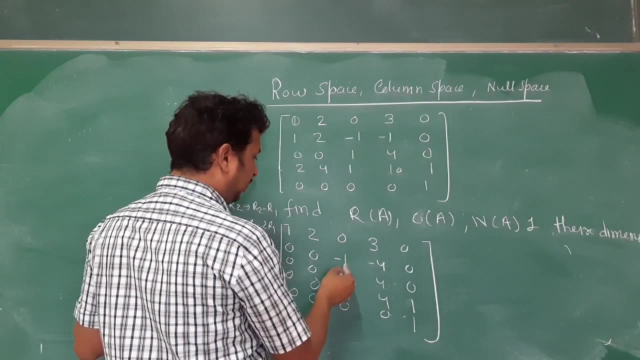 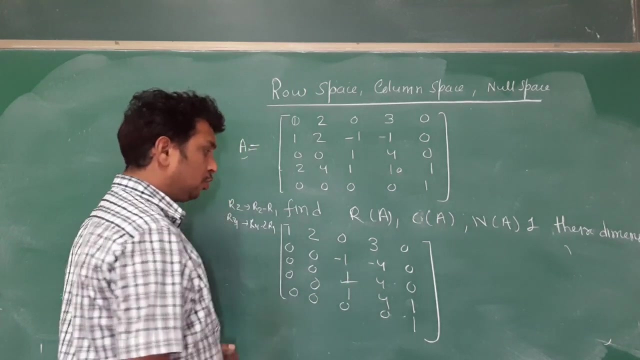 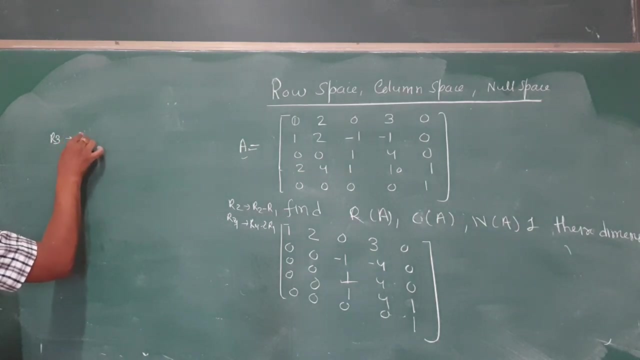 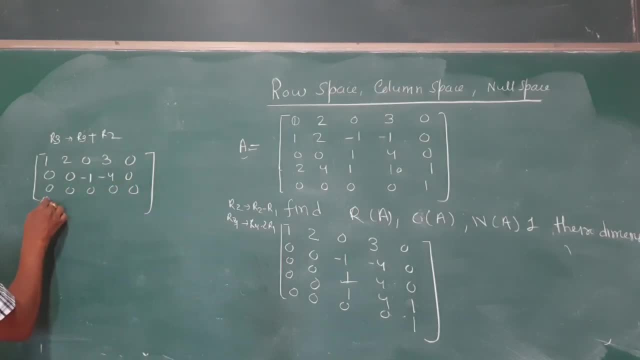 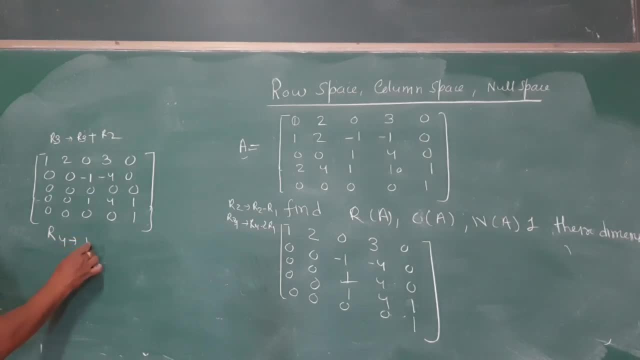 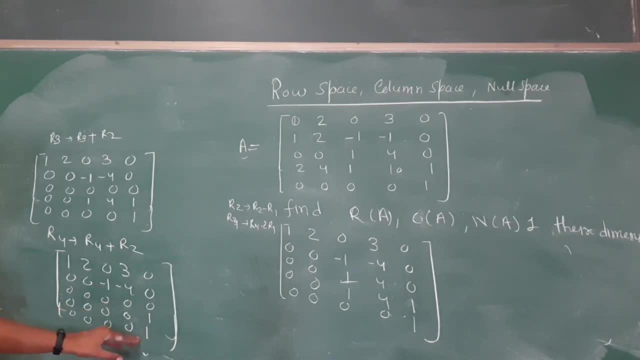 So again, if you subtract R, you go for R Y R Y minus R 4.. So what happens? 1,2,3,4,5,6,7,8,9,10,11,12,13,14,15,16,17,18,19,20,21,22,23,24,25,26,27,28,29,30,31,32,33,33,34,35,36,37,38,39,40,39,40,41,42,43,44,45,46,47,48,49,49,50,51,52,52,53,53,54,56,57,58,59,51,52,53,56,57,58,59,51,52,56,57,58,59,51,52,56,57,58,59,51,56,58,59,51,56,58,59,51,56,58,59,51,56,58,59,. 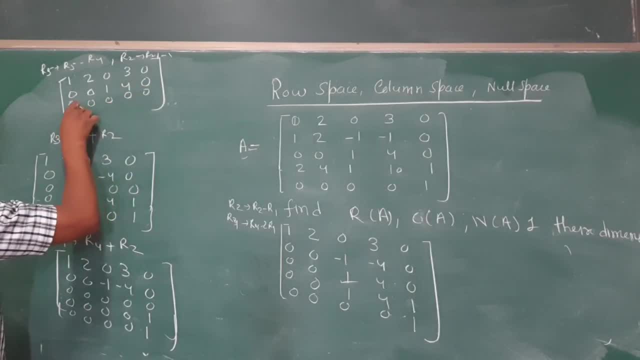 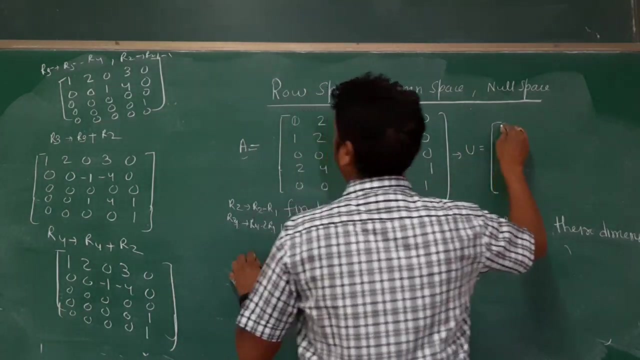 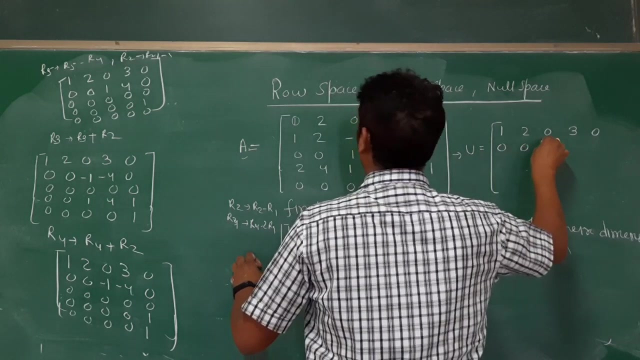 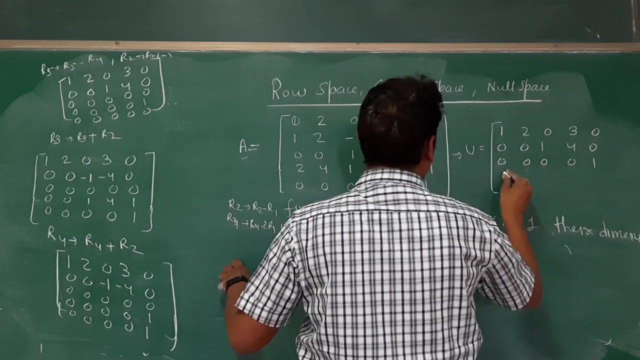 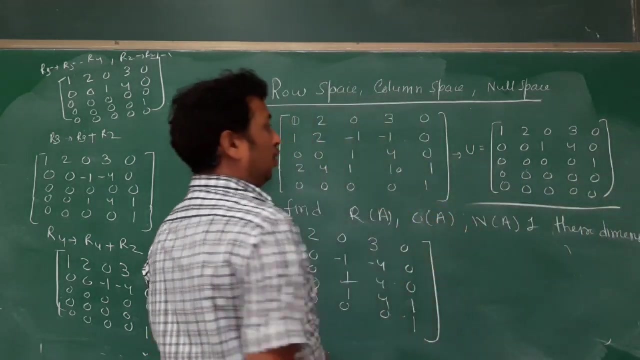 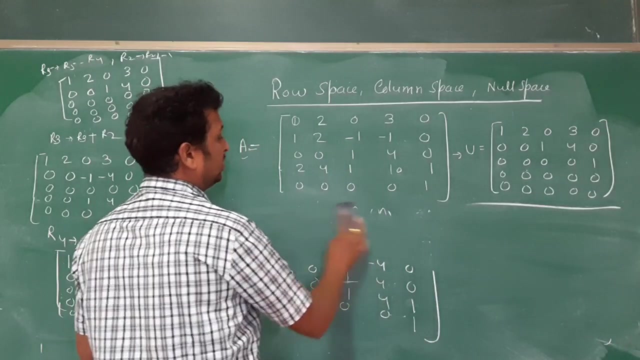 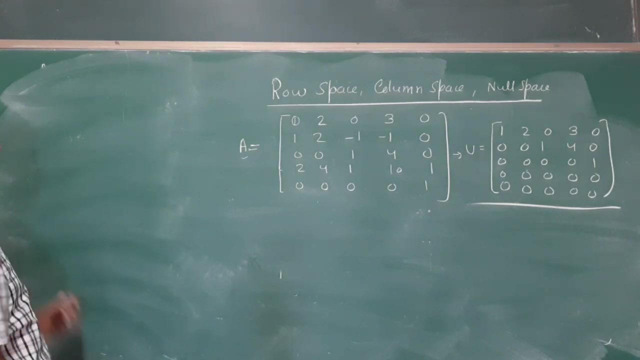 So five. What is corresponding U-magnet? Corresponding U-magnet is 1,2,0,2,0, 0,0,1,0, Then this is not 0. So this is your U matrix. Once you have U, your first step is over. Now check how many. 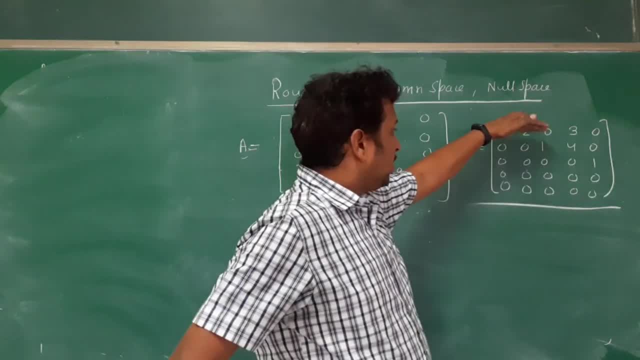 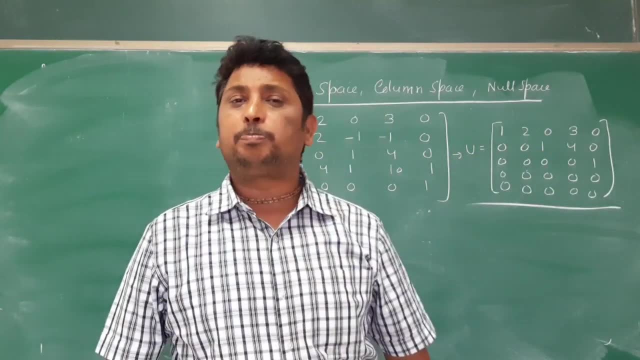 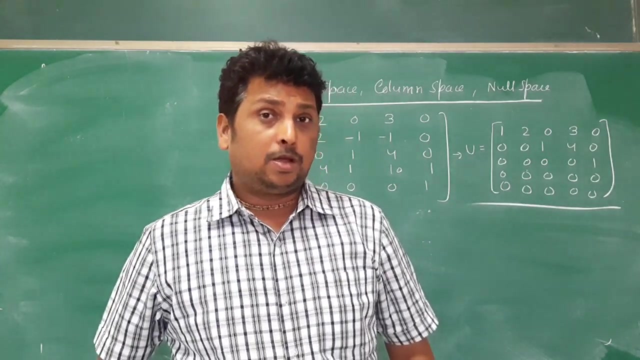 non-zero rows are there. So first is non-zero, second is non-zero, third is also non-zero. So the non-zero rows always form basis for row space. Once you converted a given matrix in equivalent form, then its non-zero rows are always linearly independent and it forms. 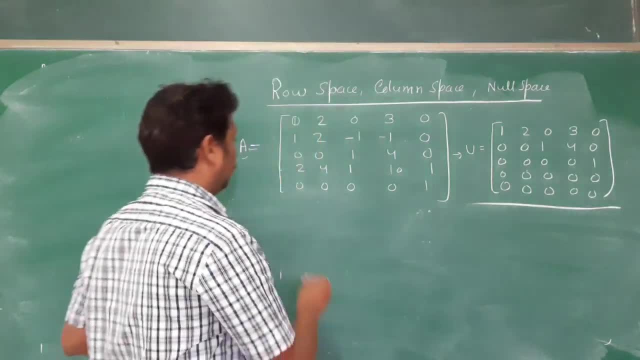 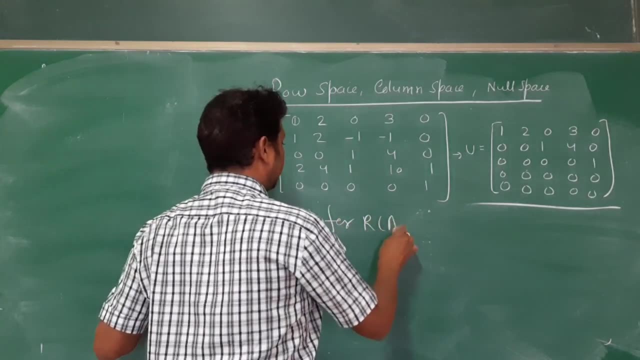 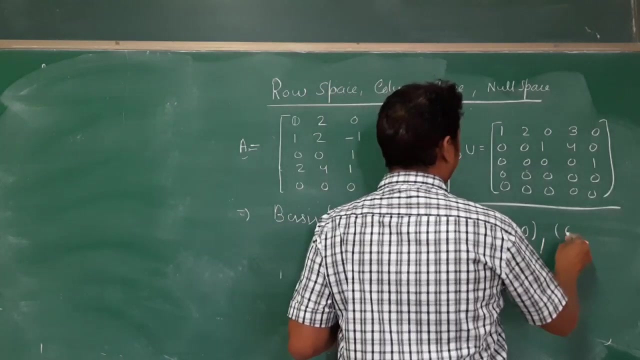 basis for row space. So what is this? Basis for RA is 1, 2, 0,, 3, 0.. First vector. what is second? 0, 0,, 1,, 4, 0.. What is third? 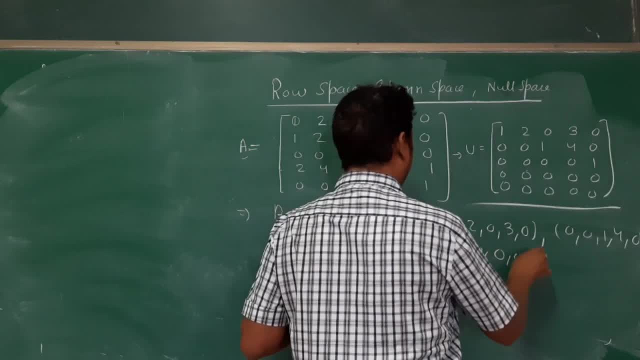 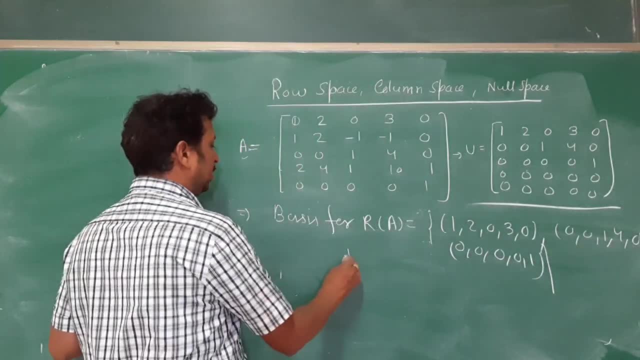 vector 0, 0, 0, 0, 0, 1.. These three elements, three rows, form basis for row space. Then what is the dimension of RA? You know very well What is the dimension: Number of elements. 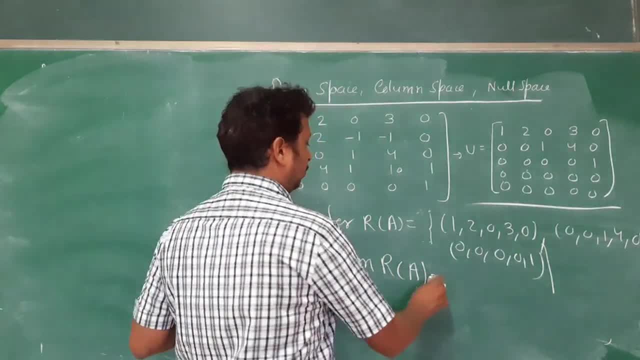 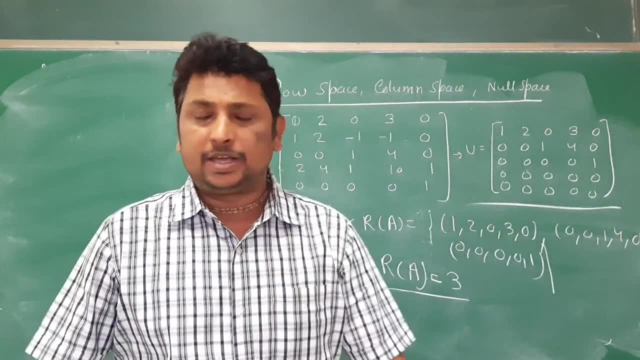 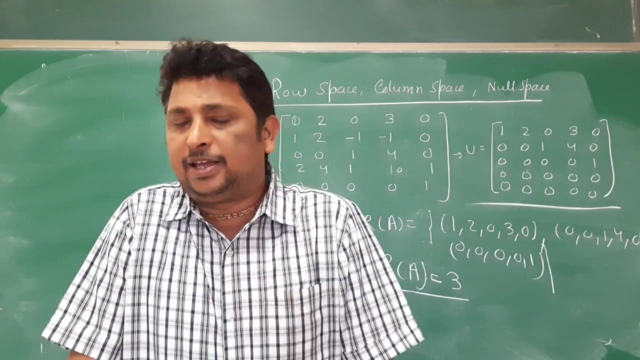 in a basis. How many elements are there? Three? So what is the dimension? So this is the way how we calculate row space. Understand It is very easy: Just convert the given matrix into equivalent form and then check how many non-zero rows are there. Write that one That. 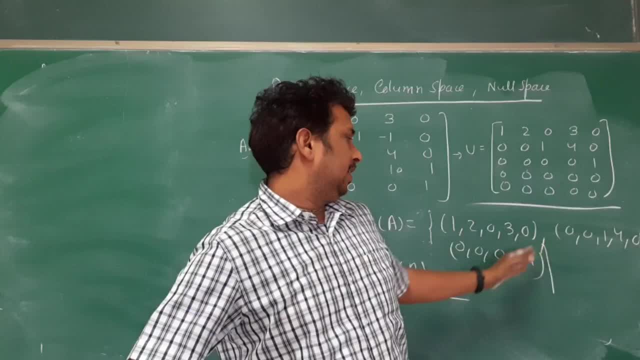 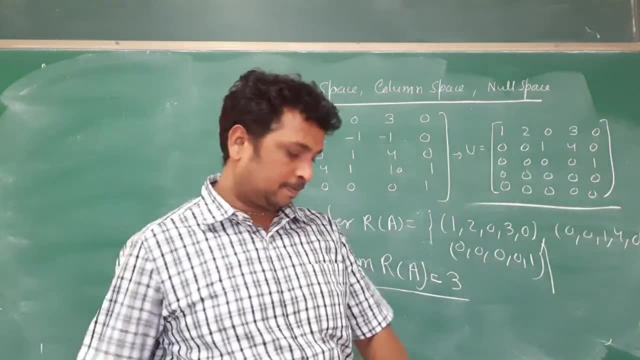 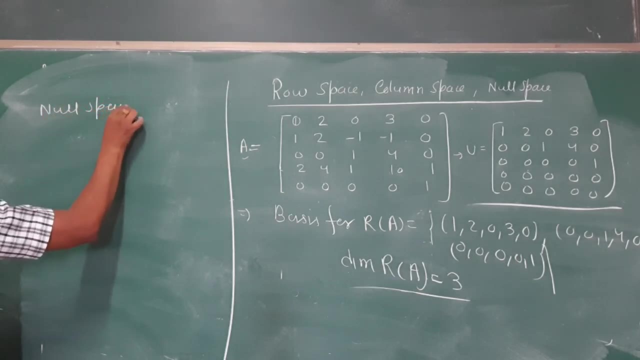 forms, basis. So what are the basis elements, These three, And what is the dimension Three? So in this way we calculate row space. Now I am going to explain about null space, How we calculate null space. Null space means solution of G, y to the. 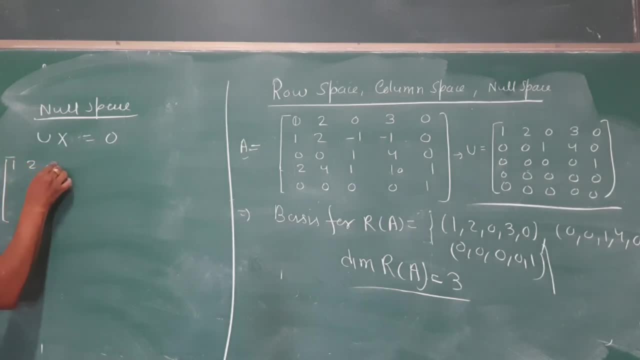 root of z is equal to 0.. What is u? What is x? See this. what is the order? 5 goes, I mean comes 5.. This is also 5 required. So x1 equates with 0, 0.. So sometimes we have to find these values. 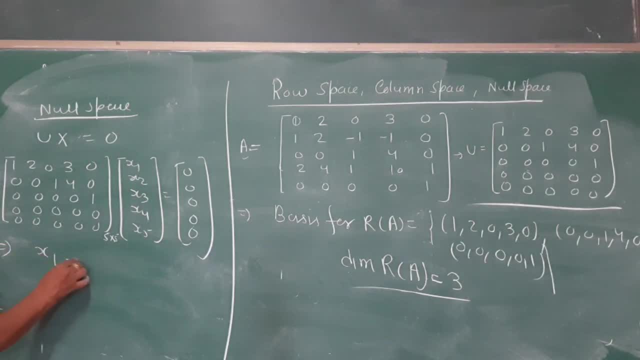 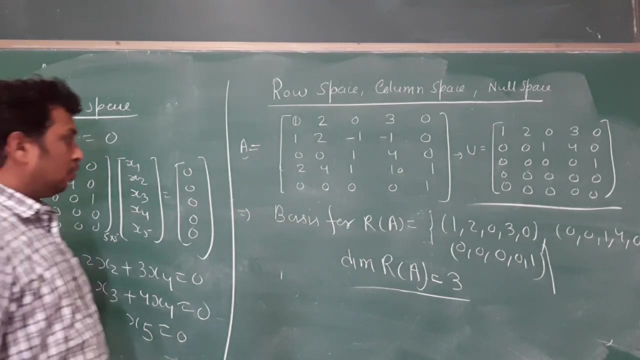 So write in my equation, for x1 plus 2x2 plus 3x4 is equal to 0. Then x3 plus 4x4 is equal to 0. Then x5 is equal to 0. So now, once you know it, 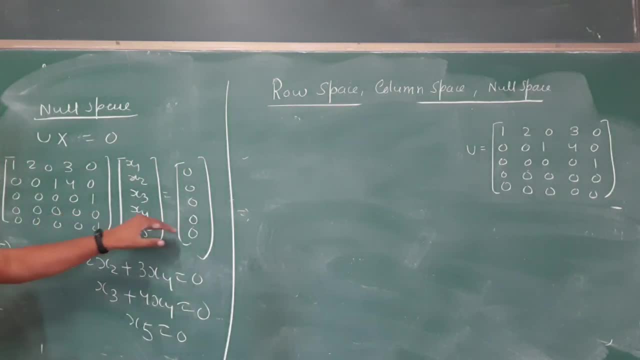 you multiply this and it will show: See 3 equations. So already x5 is 0. So we have actually 3 equations, 5 unknowns. So 2 variables you have to choose by yourself. Remember we have 3 equations and 5 unknowns. 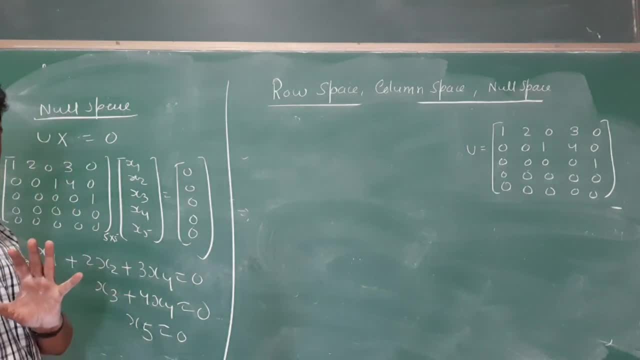 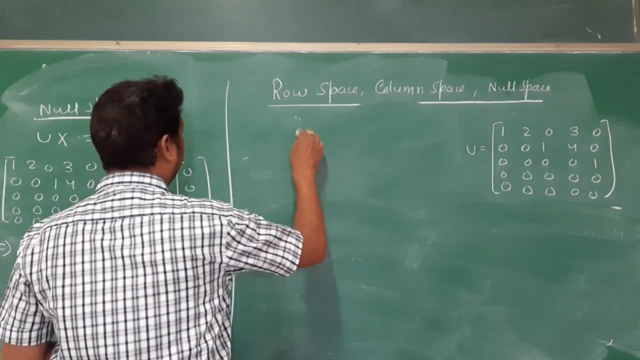 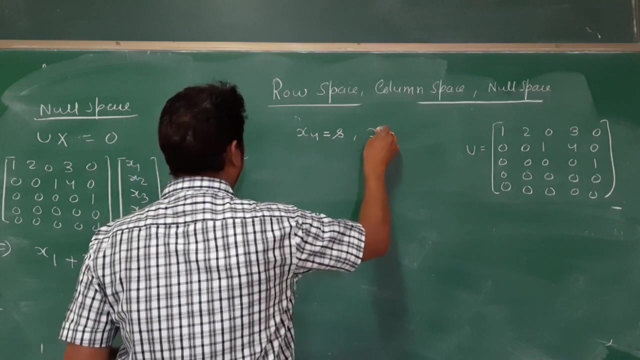 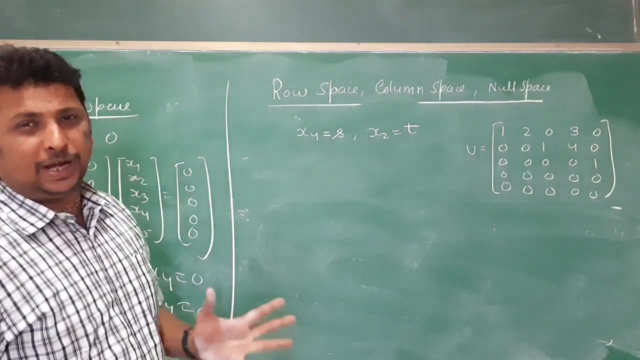 We have to choose 2 variables by ourselves, Because x1, right, So x1, we take by ourselves. So we take x4 is equal to s and x2 is equal to p. Your choice, You can choose your way. You can choose x1,, x2,, x3,, x4. 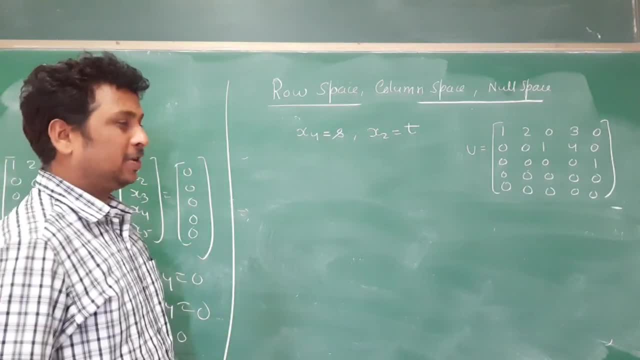 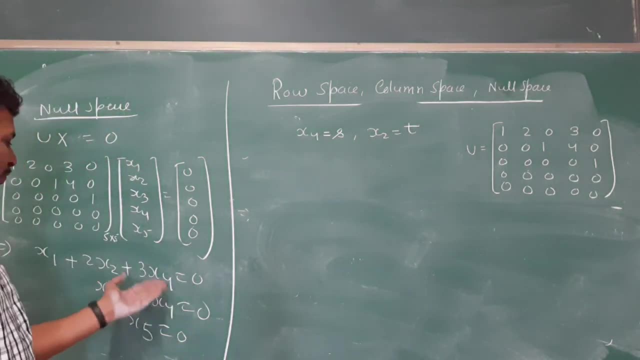 x5 parallel is 0. So don't choose that one Because it does not look good. Otherwise, your choice. You can do whatever you want, But don't choose x5.. Go for this one. In other cases you choose x5 as well. So x4 has x2, p. 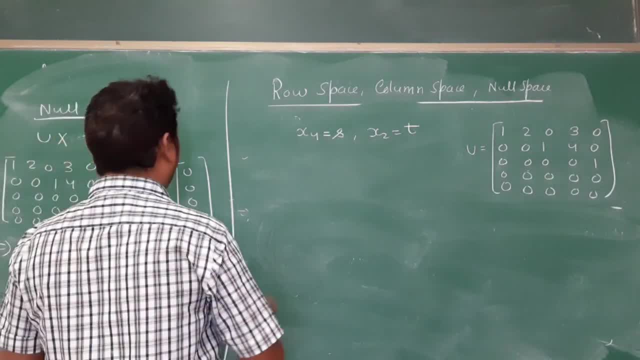 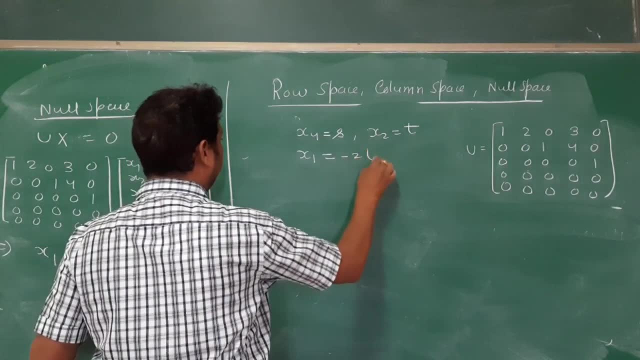 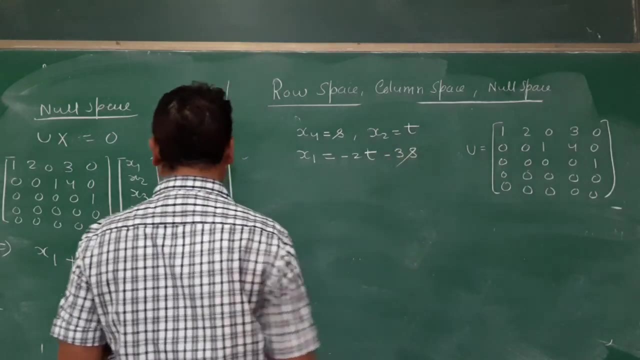 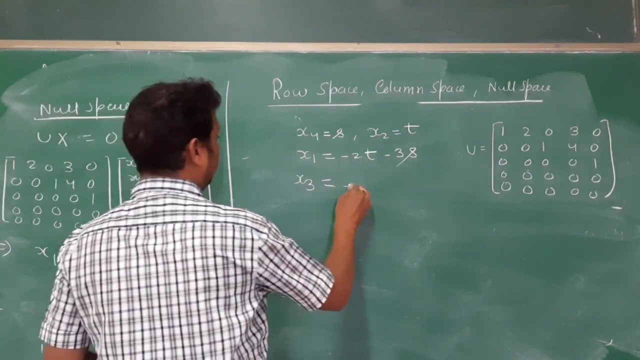 What is x 3 values? So what is x1?? x1 is minus 2x2.. This is minus 2p. Plus 3x1 is minus 3x2.. What is x3 value Minus 4x2.. This is minus 4x. 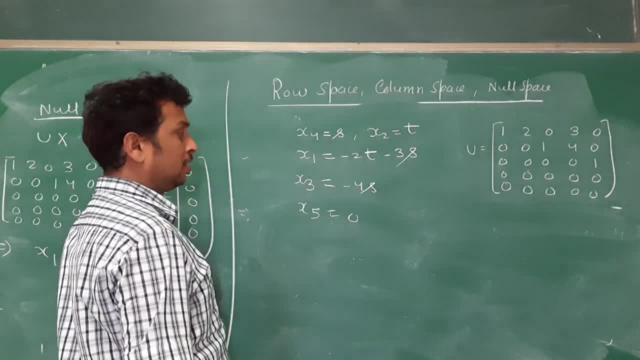 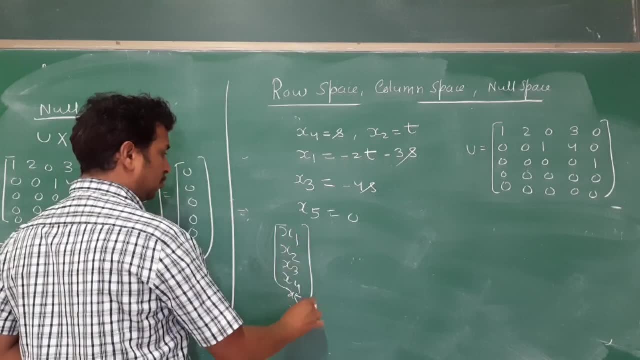 What is x5 value? So we calculated all values. So what is assumption? We have x1, x2, x3, x4, x5.. So write What is x1?? x1 is minus 2t, minus 3s. 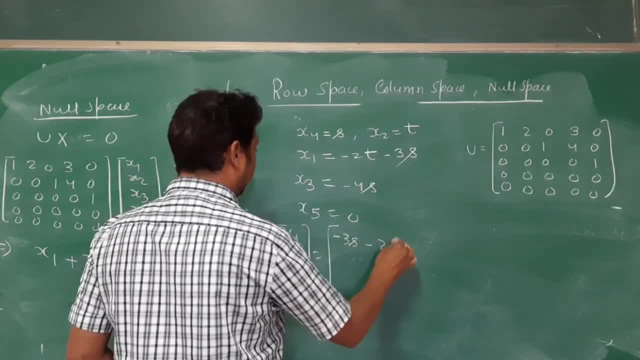 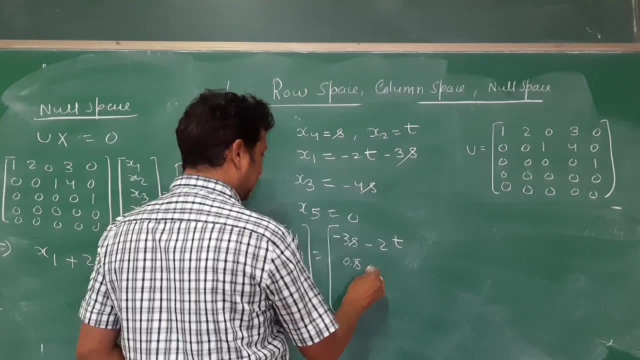 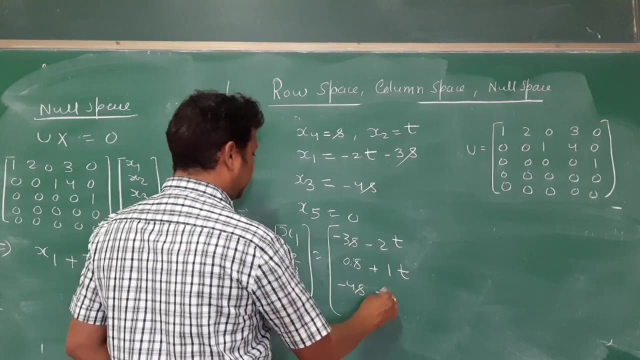 So minus 3s Minus 2t, What is x3?? x3 is t. t means 0s plus 1t, Correct: What is x3?? Minus 4s plus 0t, What is x4?? 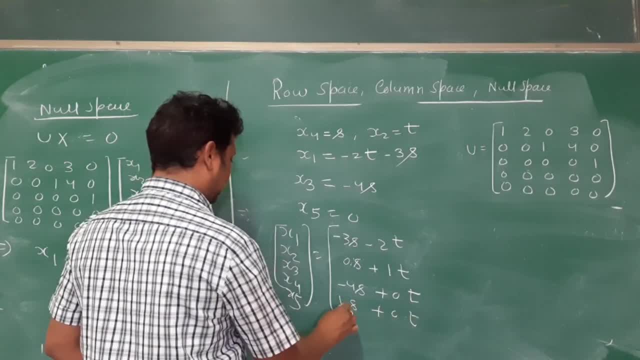 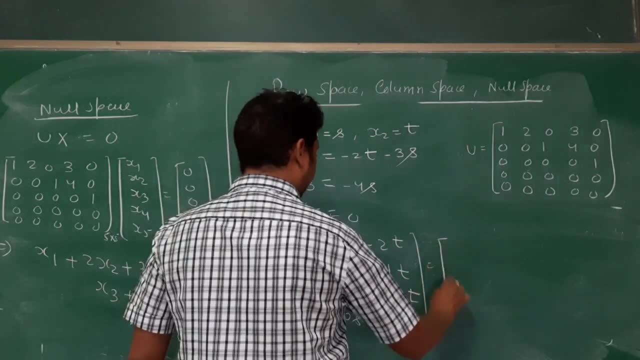 s plus 0t, What is x5?? 0.. 0 plus 0. 0s is 0t. Separate s with s, t with t. So what is the difference Minus 3. 0.. 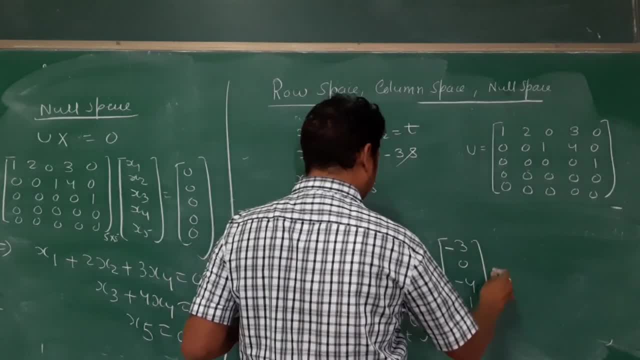 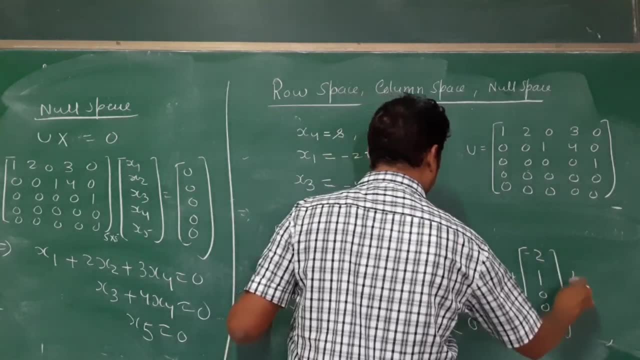 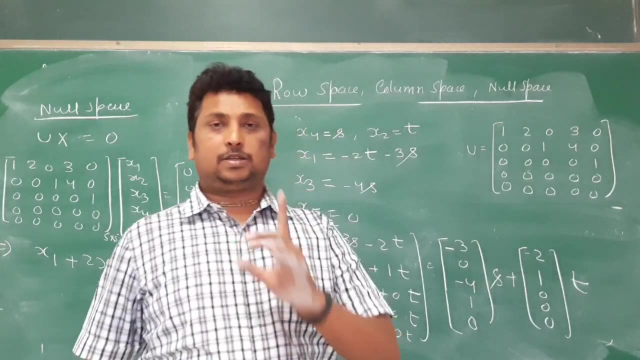 Minus 4. 1. 0.. This is multiplied with s Plus 40.. Minus 2. 1. 0.. 0.. 0.. Over The coefficient of s and t forms basis for null space. 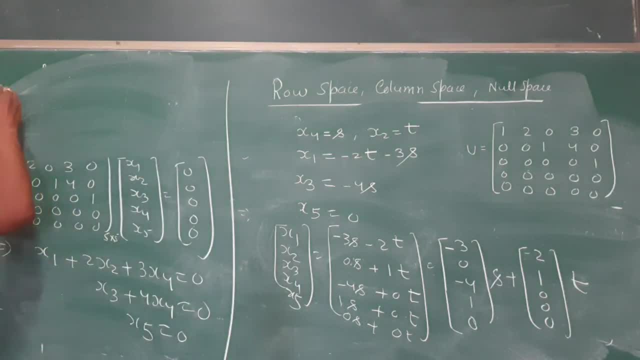 So what is the basis for null space? Minus 3. 0.. Minus 4. 1. 0. And minus 2. 1. 0. 0. 0. These two elements form basis for null space. 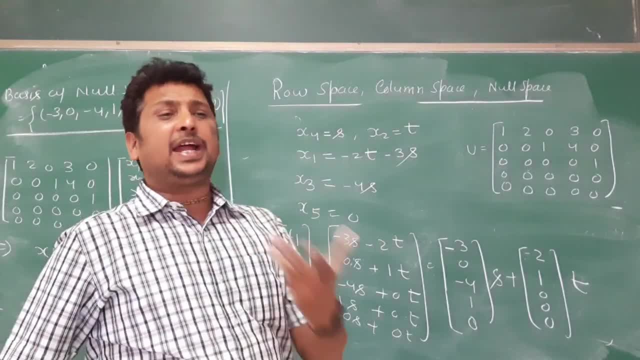 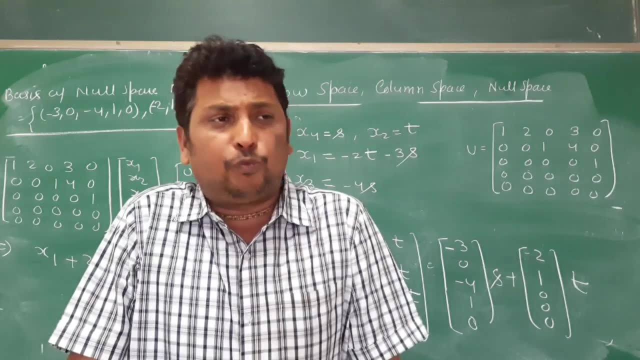 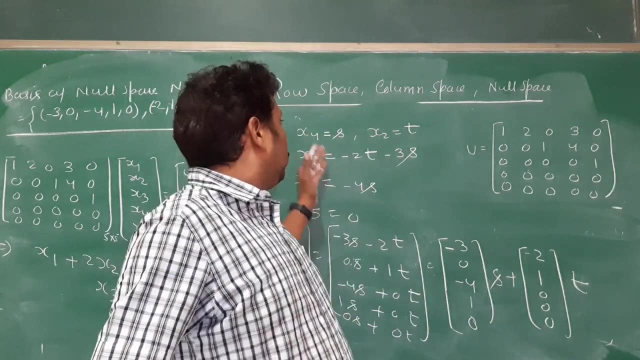 So how many equations are there? How many x's are there? Take any two: s and t. If it is two more than Otherwise, if one more than then, only take s And write. in this way You will find out all values in terms of s or t, or only s or only t. 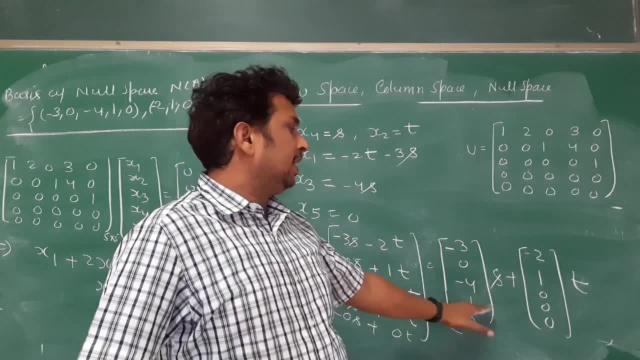 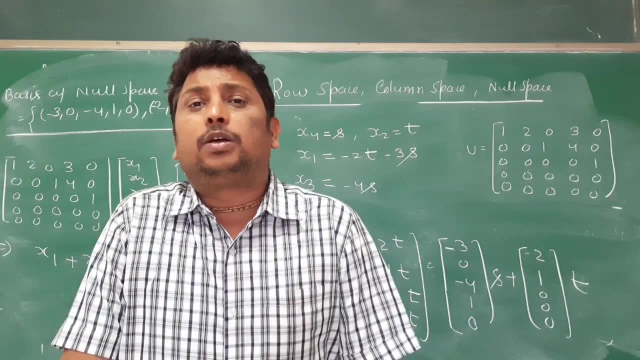 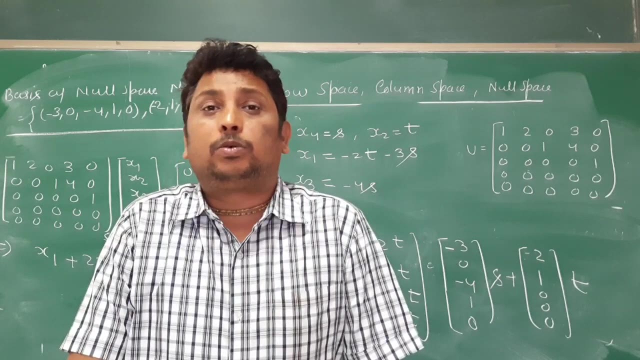 Your choice. So once you have calculated, converted in this way, the corresponding coefficient is your space. That is called null space, So null space basis. once you know, you can easily write what dimension of null space That is 2. there Now you can verify. 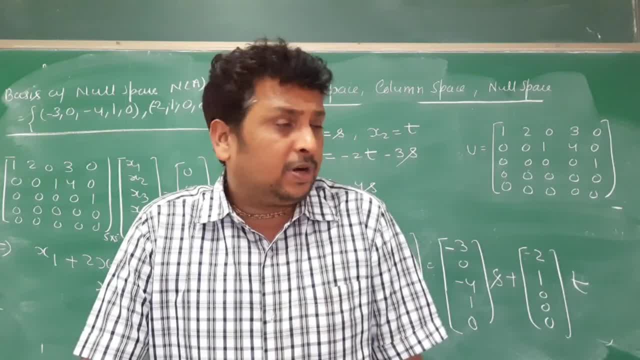 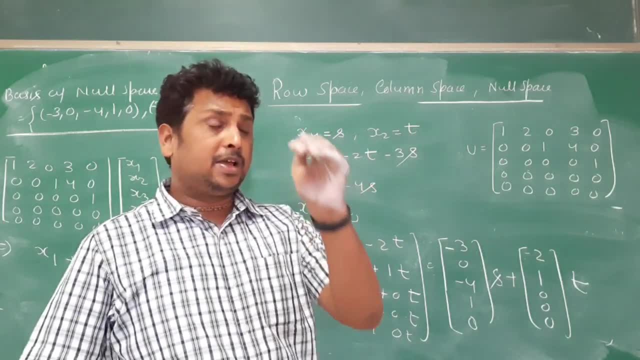 What is the dimension of matrix? 5. What is the dimension of row space? 3. So rank-null theorem applies there. It means rank of matrix plus null space of matrix. Dimension of null space is equal to order of matrix. What is the order? 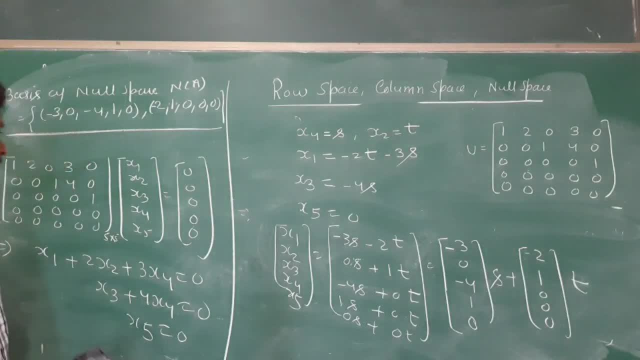 5. What is positive? case Letter m: Letter m: Remember: 1 comma 1 comma plus 1.. Okay, so you can write What is the part you are going to calculate: 2 comma, 2 comma 3, because we knew it hosted together. 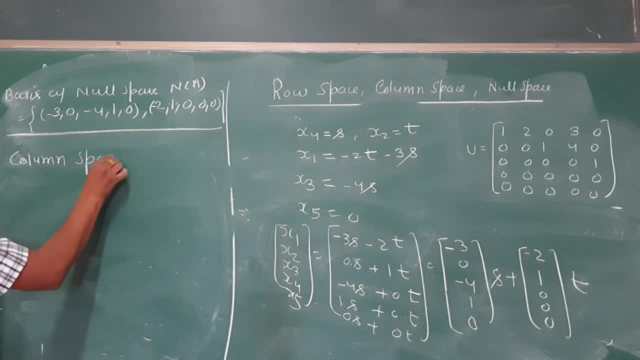 This is called positive case for letter m Love now size. now write: Is this vector. write the take c1, c2, c3,, c4, c5 and write the equation form using null space. So what we get minus 3 is c1, minus 4 is c4, what we write plus 0 is c2, minus 4 is. 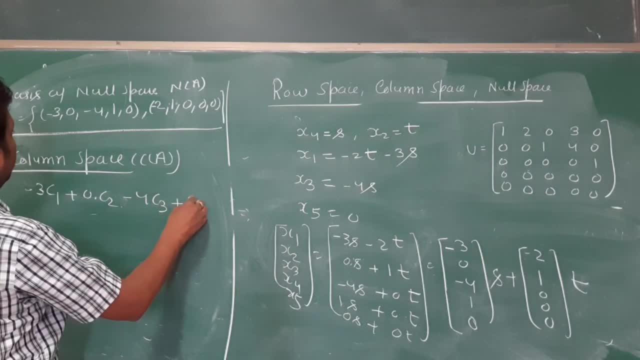 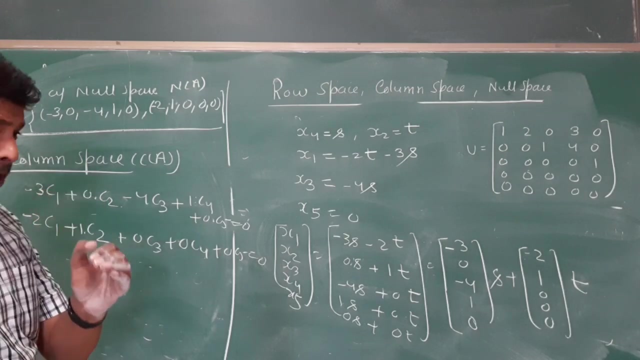 c3, plus 1 is c4, plus 0 is c5 is equal to 0.. For second: minus 2 is c1, plus c2, 1 is c2, plus 0 is c3, plus 0 is c4, plus 0 is c5 is equal to 0.. So see which variables. 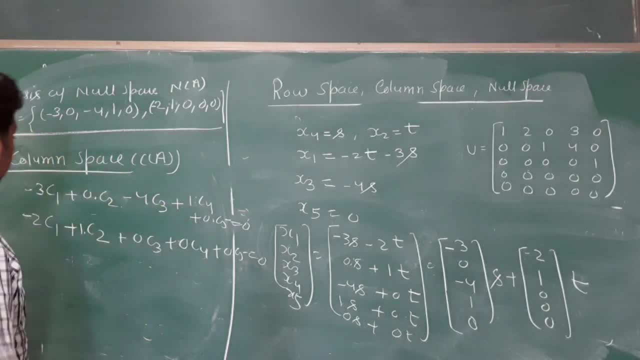 forms identity matrix out of these five. So see C4,. what is the question? 1 and here 0, that is okay. Now one more, c5, where 0 is c2, 1 and here 0, correct. So c2 and c4 forms identity matrix, correct or not? C, you write. 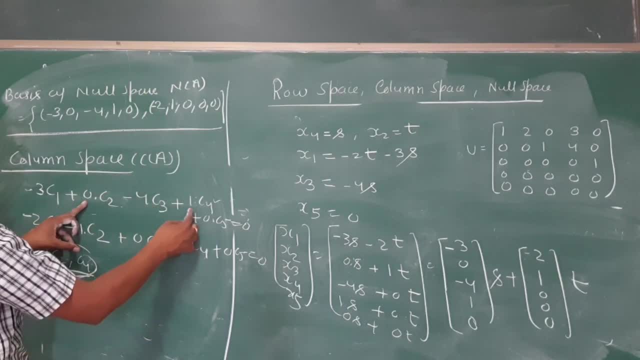 c4 first, So 1, here in this equation, 0, here is 0, here is 1.. So this forms identity matrix. So remove this, So remaining so columns. What are the columns remaining This? 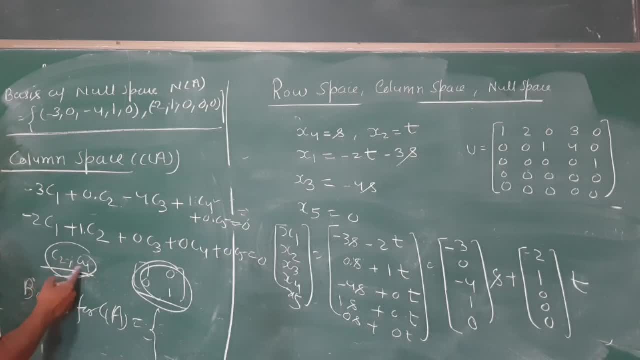 is called column, space is remaining column. Whatever forms identity matrix, that is three variables. remove it, What is remaining? Different variables- and then what is remaining c2, c4 over c1, c3, c5.. So c1, c3, c5.. 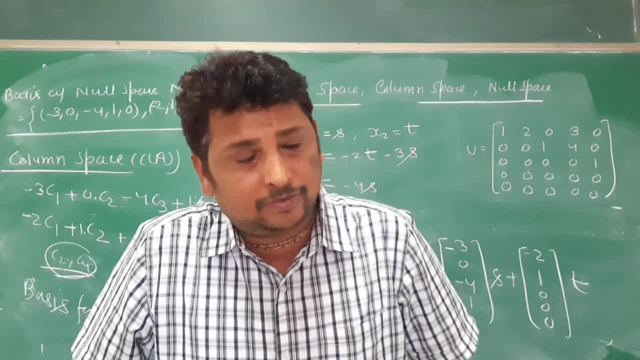 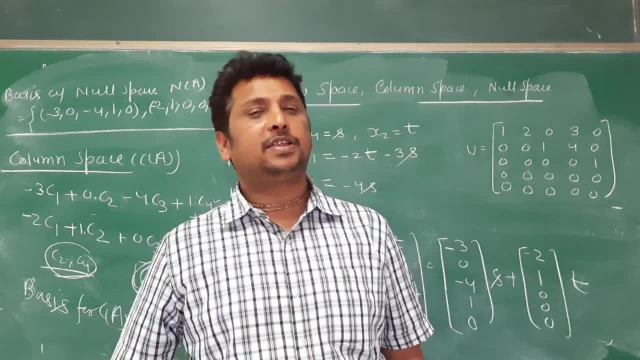 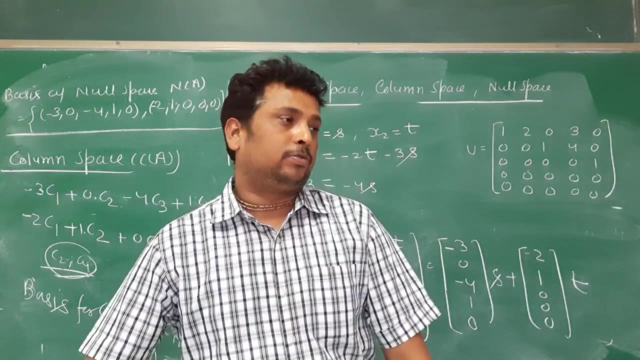 These three columns of the given matrix forms the column space. So what is the dimension 3.. So hope you understand this. This is very important how we calculate row space, column space and null space of a given matrix. So please do it and please subscribe the channel. 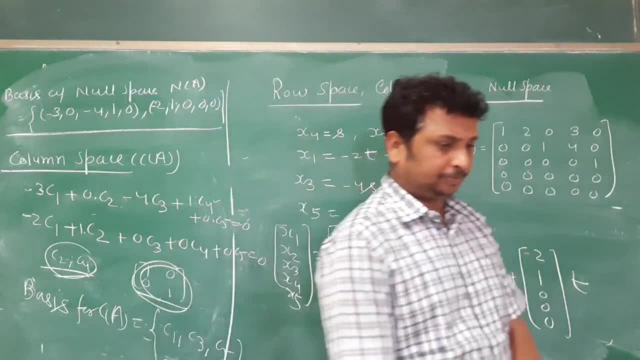 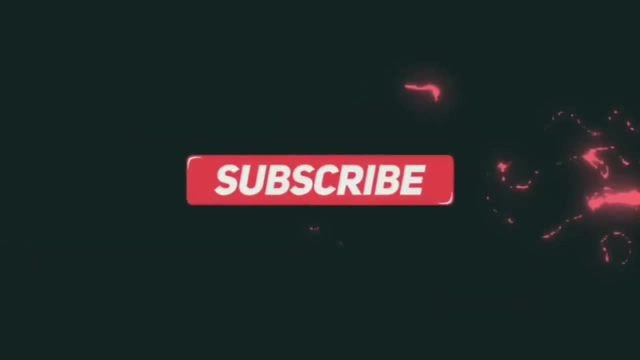 That is also very important, Thank you. Thank you very much.